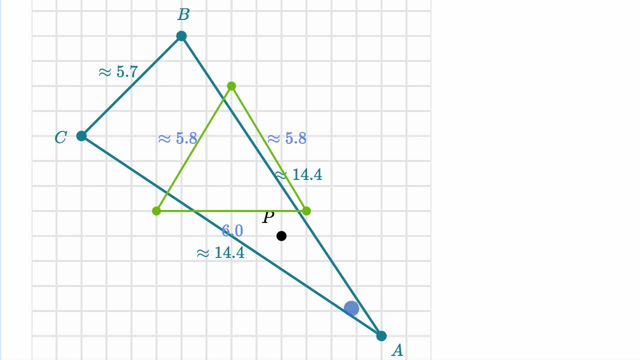 we can see that we are crossing one square, two squares, three squares, four squares. So if we have a scale factor of 1, 4th, instead of crossing four squares diagonally, we would only cross one square diagonally. So I'll put the corresponding point to A right over there. 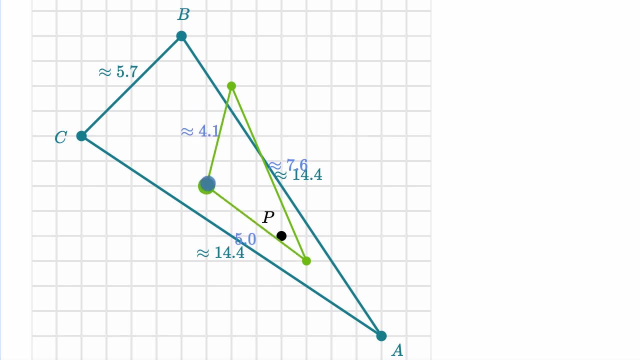 Now, what about for point C? It's not quite as obvious, but one way we could think about it is we could think about how far are we going horizontally from P to C, and then how far do we go vertically? So horizontally we're going one, two, three, four. 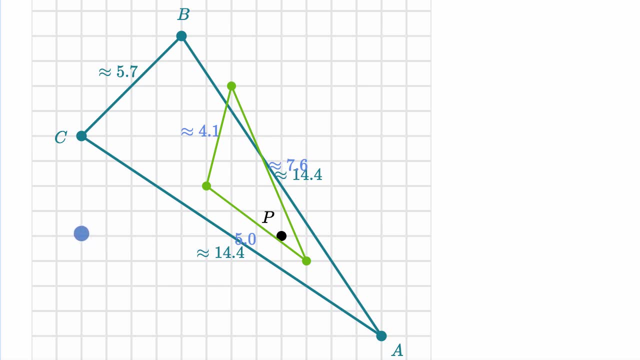 five, six, seven, eight of these units, And then vertically we're going one, two, three, four. So we're going to the left, eight and up four. Now if we have a scale factor of 1, 4th, 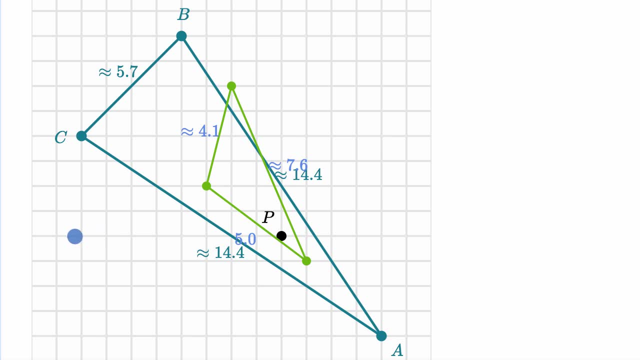 we just multiply each of those by 1- 4th. So instead of going to the left eight, we would go to the left two. Eight times 1, 4th is two. Instead of going up four, we would go up one. 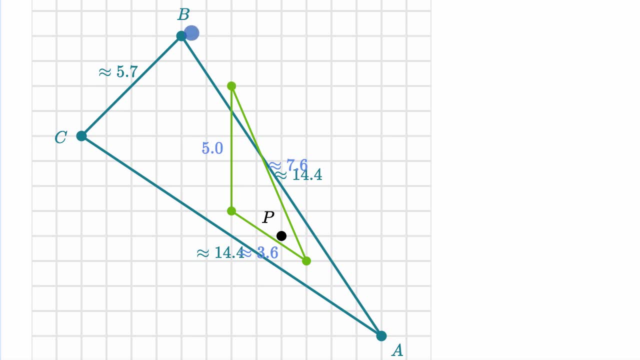 So this would be the corresponding point to point C, And then we'll do the same thing for point B. When we go from P to B, we're going one, two, three, four, five, six, seven, eight up. 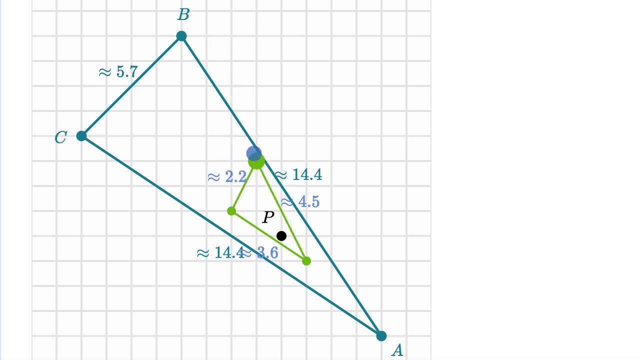 and we're going four to the left. So if we have a scale factor of 1- 4th, instead of going eight up, we'll go two up, and instead of going four to the left, we will go one to the left. 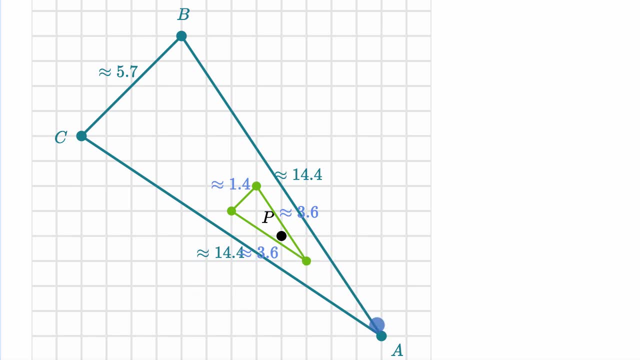 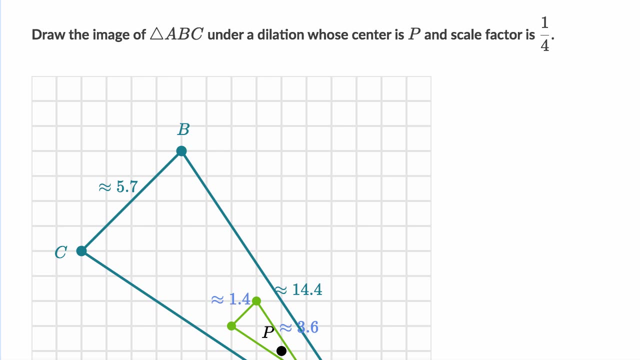 So there you have it. We have just dilated triangle ABC around point P with a scale factor of 1- 4th and we are done, Thank you. 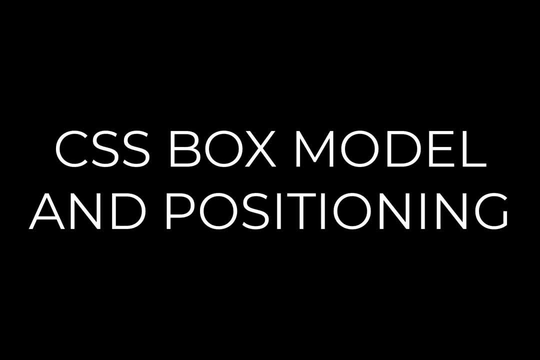 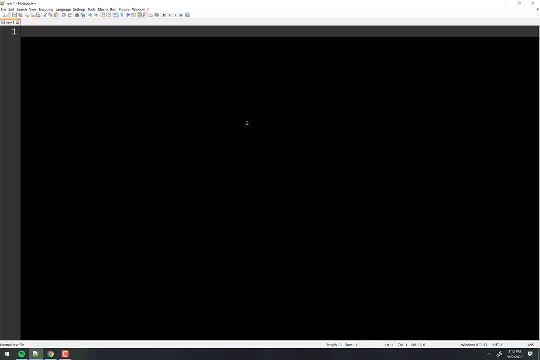 CSIS 1430 is filmed before a live studio audience. All right, so what we're going to be talking about today is a couple things: Box model and then positioning. The box model is tricky business and positioning is trickier business, And part two of positioning is trickiest business of all. right.